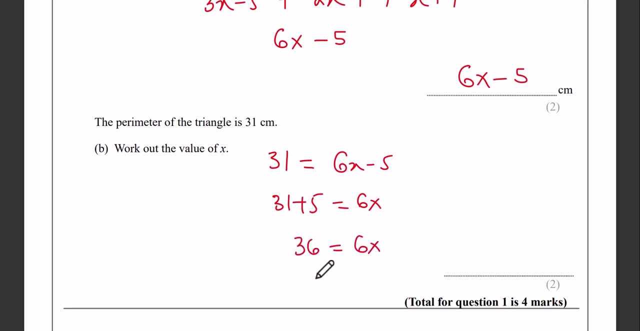 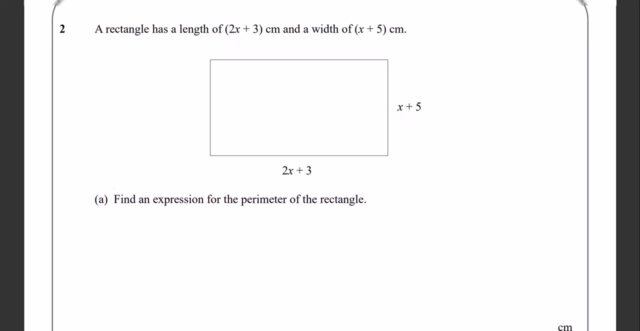 And this equals to 6x, and I'll divide this by 6,, definitely x will be 6.. So the value for x: x6.. Now you can do the same for the next question. yeah, because this question here we have a side, 2x plus 3 and x plus 5, and this is a rectangle. 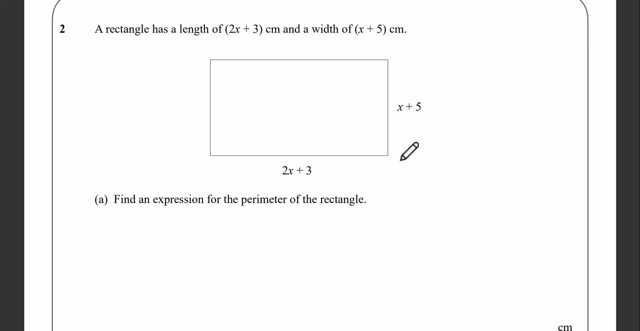 And so we want to work out for the expression for the perimeter. So I do know that if it's x plus 5, definitely here, Here, it has to be x plus 5.. If this is 2x plus 3, that means the top has to be 2x plus 3.. 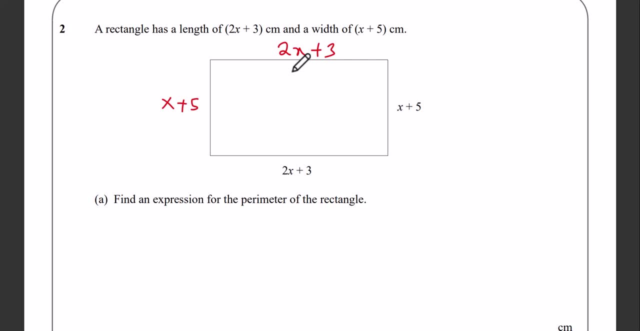 That's because this is a triangle. I mean a rectangle, right? Good, So now, if you add up all the sides, x plus 5 and x plus 5, and here which is 2x plus 3, and the top is also 2x plus 3.. 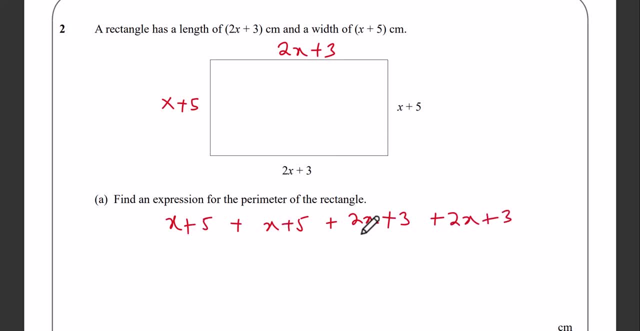 Now, if you add up the left, So in terms of x and x is 2x, plus another 2x plus 4x plus 2x, I think that's going to be like 6x. And now you add the numbers, and 5 and 5 is 10 plus 3 is 13 plus 3 is 16.. 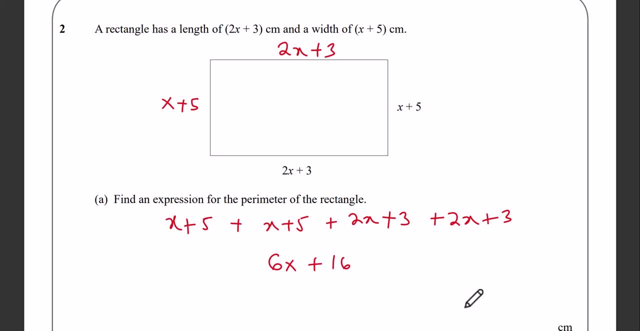 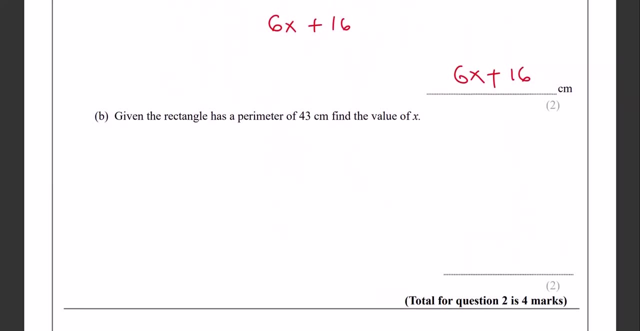 So an expression for the perimeter in terms of x is 6x plus 16 centimeter, And you can work out the. now we told that the rectangle is 43, right, And so we need to work out the value of x. 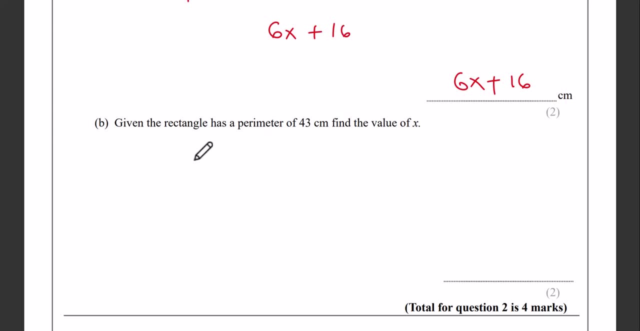 Okay. So I think what we need to do is use our perimeter, which is definitely going to be 43, with the expression in terms of x is 6x plus 16.. Now what you do? you subtract 16 on both sides. 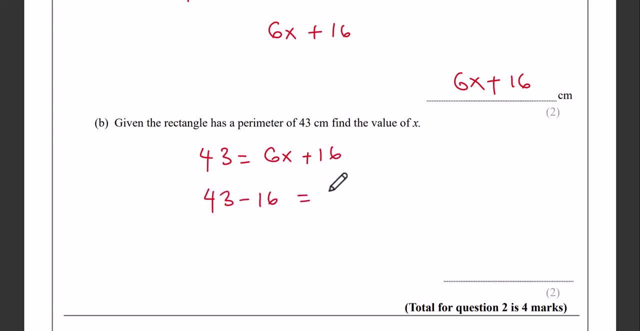 So you have 43 minus 16, and it's equals to 6x. Okay, So if you subtract this, you get 27,, and that's equals to 6x. So x is definitely going to be 27 divided by 6.. 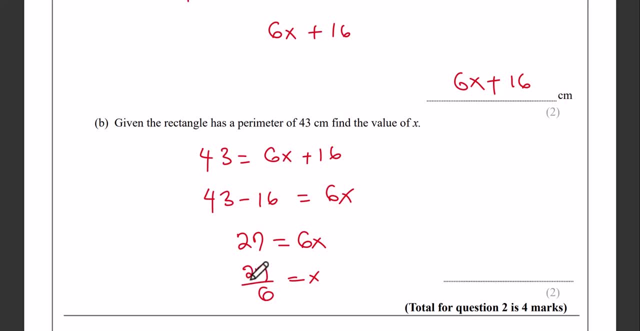 That's x, And if you cancel it out, 27 definitely has to be like 9, and 26 has to be 2.. And, of course, if you divide this it's going to be 4.5.. So that means x is definitely going to be 4.5. 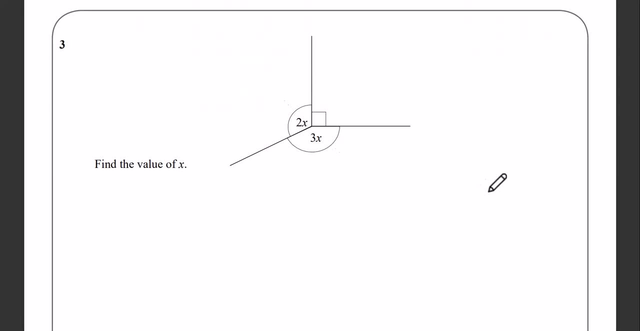 And then we go to the next question. Okay, So we have the values of x, Here is 2x and here is 3x and here is just 90 degrees, and we need to work out the x. 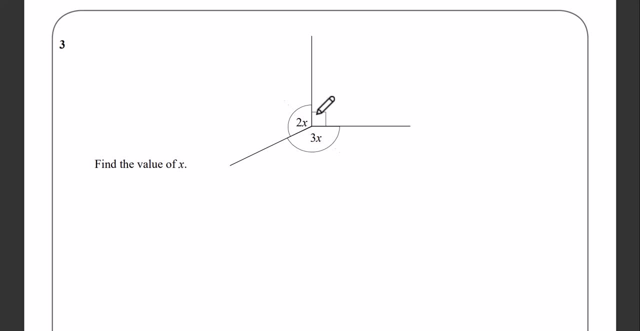 Now this is trying to add up all the sides, which is going to be 360.. So you add 2x plus 3x plus 90 degree And, of course, if we add up the angles around the point, it's going to give you 360 degrees. 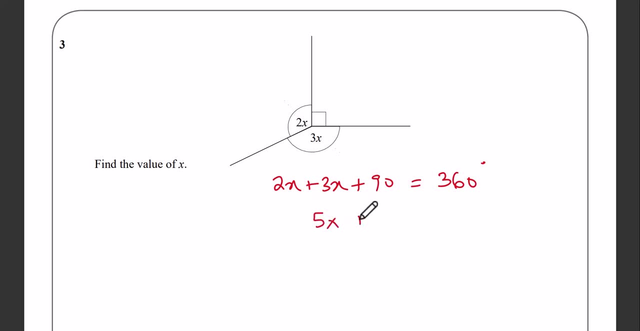 Okay, Now, if you add, this is 5x plus 90, and it's equals to 360.. And of course you're going to subtract 90 on both sides, So that's going to give you like 270. 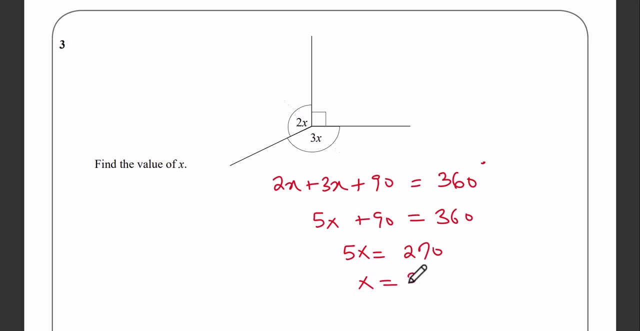 And, of course, to get x, divide by 5.. So divide 270 by 5. And I think the answer will be so, if you divide the answer it's going to be 54.. All right, So x is 54.. 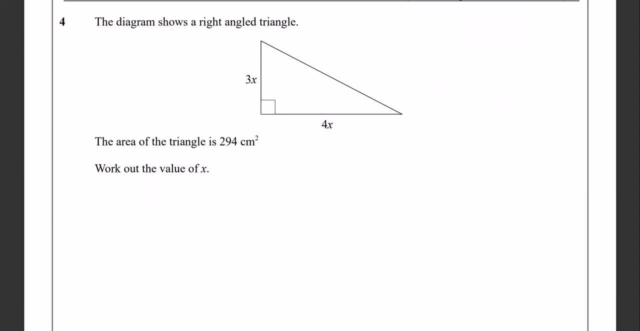 And now we go to the next question. We have a, we have a um, A dash, We have a diagram that shows a triangle and the height is 3x and the bottom is 4x, And we also know the area, which is going to be 294 centimeters squared. 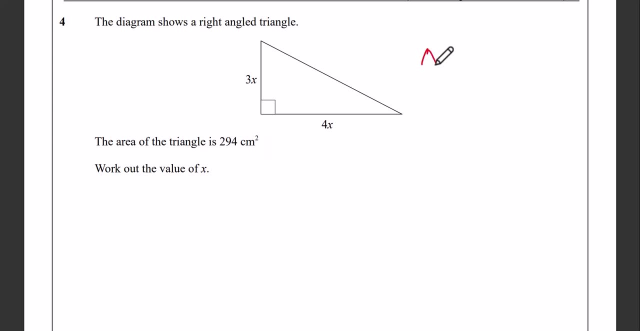 And you want to work out the value of x. Now, the area of a triangle is given by the formula of the base times height. and you have it, And already you know the area, which is going to be 294.. And the base is already 4x multiplied by the height, which is 3x. 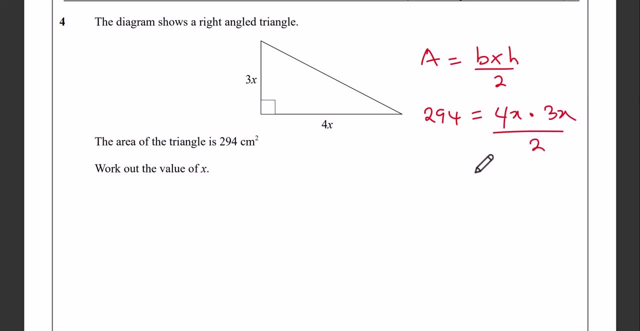 And you have your answer. Of course, if you multiply 3x and 4x, you get 12x squared And divided by 2.. And if you have 12 by 2, that's going to be 6x. 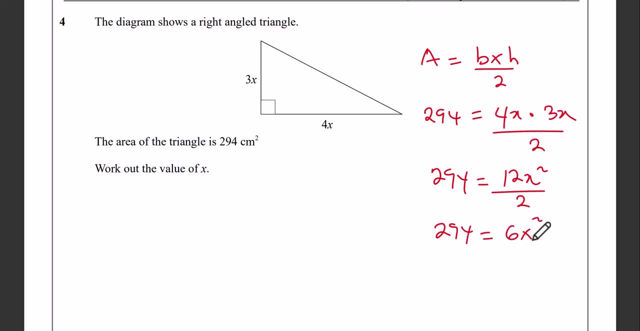 So 294 is 6x squared, And now you divide both sides by 6. And that means, um, That's going to give me 294 divided by 6.. 294 divided by 6.. Equals x squared, okay. 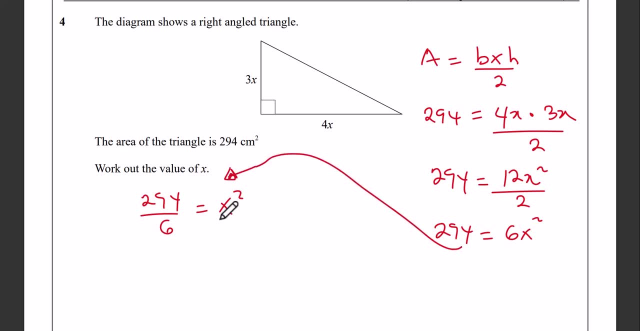 So I have to bring this in here. okay, That's where it works. So you divide 294 by 6.. So if you divide by 6, you get 49.. And x squared, And so to get x, you do the square root of 49, which is definitely going to be 7.. 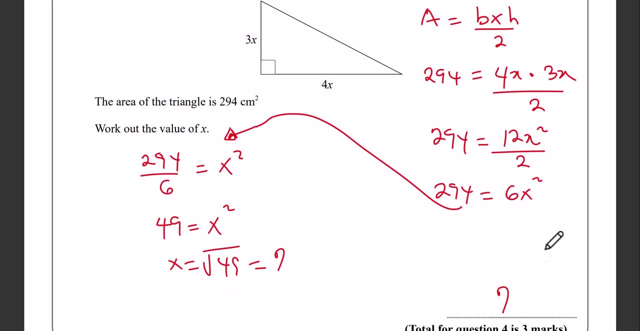 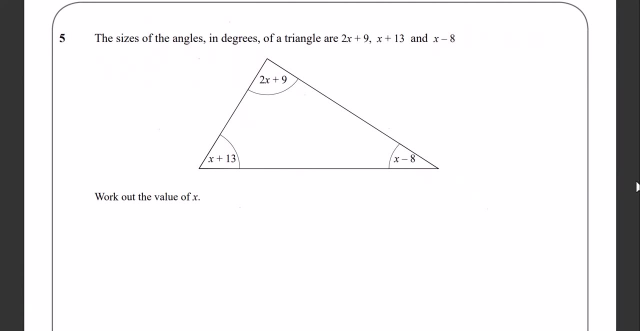 So x is definitely going to be 7.. So, and we come to the next question. here We have a triangle and all the angles are all given And we need to work out the angle x. You know, when you add up all the three angles you're going to add. 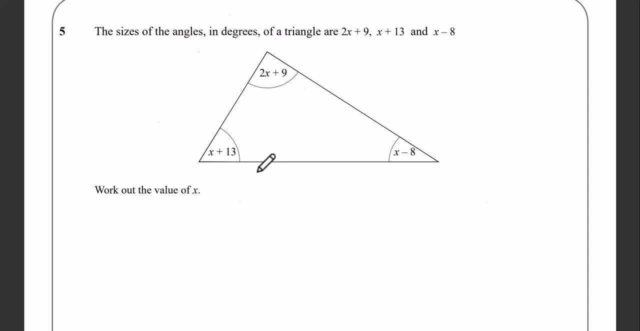 You get 180, right? So if you add 2x plus 9 plus x plus 13. And then, of course, you add x minus 8. If you add all three angles, you're going to be given 180.. 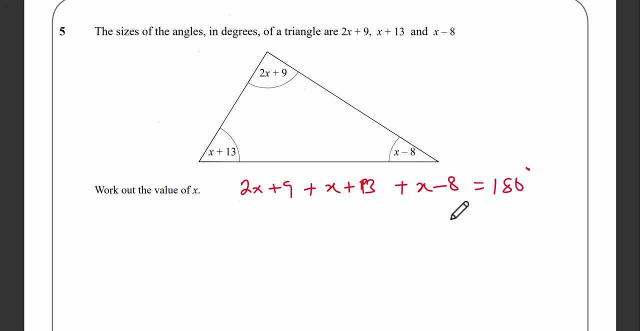 Because the sum of angles in a triangle is 180. So you add up the x's, That's going to give you 3x plus 1x is 4x, And add up the x- 9 plus 13,, which I think is going to be like 22.. 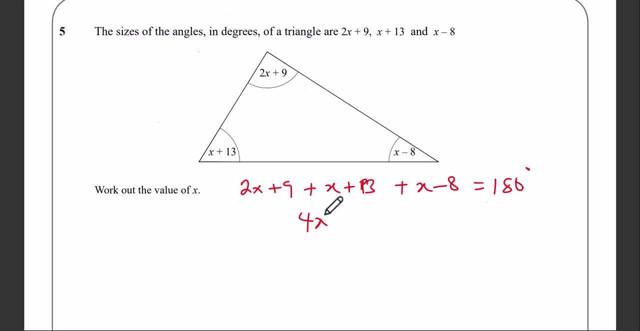 And 22 take away 8.. It's going to give you minus 14.. All right, so I'll just give you plus 14,, okay, And this is equal to 118.. And, of course, you have to separate 14 on both sides. 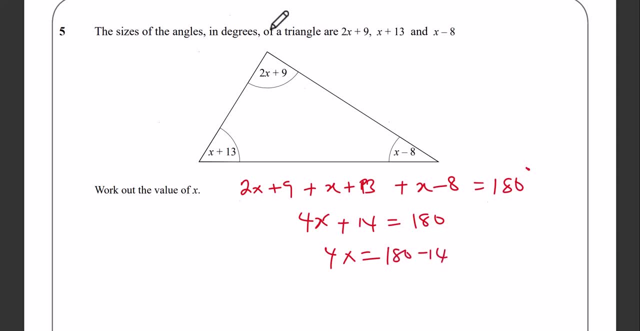 So 4x is equal to 180 minus 14.. I think that's going to give me something like That's 166.. So 4x is 166.. Now I don't have enough space here. Okay, I think I have some space. 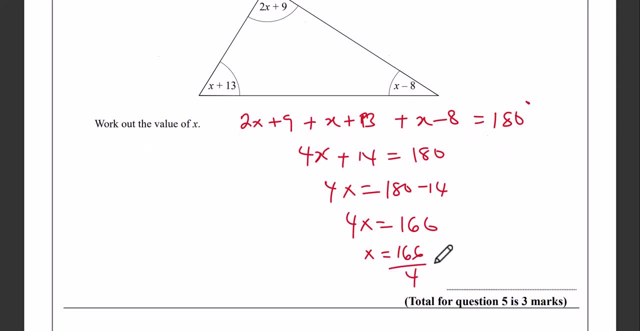 And divide both of them by 4.. So 166 divided by 4. I think the result will be: And that will be like 41.5.. I think so, Yeah, 41.5.. Now we go to the next question. 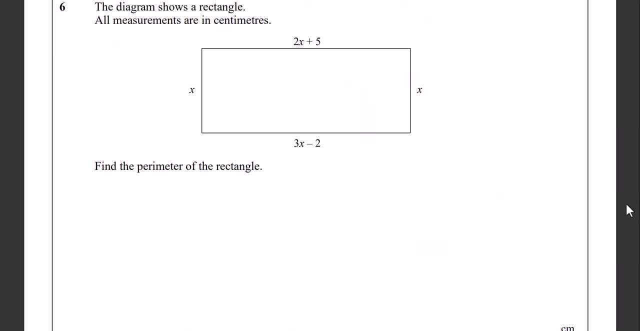 We know the diagram of a rectangle or measurement of centimeters, And you have to work out a parameter. All right, so this side and here are the same. Of course, this side and here has to be the same, But you need a numerical value for this parameter. 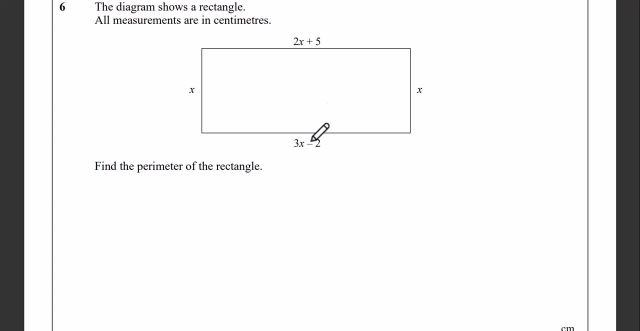 So I think what I needed to do was to take: here is equal to here, So that's 3x minus 2 is equal to the top, which is 2x plus 5.. And of course, I can subtract 2x on both sides. 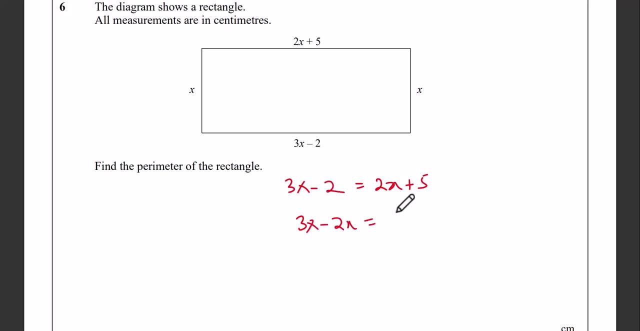 So that's 3x minus 2x And add 2 on the other side, That's 5 plus 2.. And of course it's going to give me x, And 5 plus 2 is 7.. 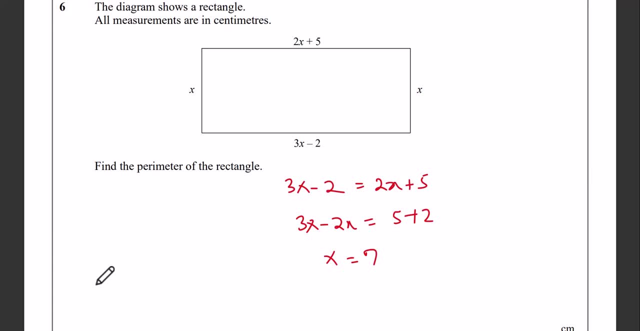 All right, Good, Now to find the parameter. Now the parameter has to be: You have to add up all the sides, But first I think I need to work out what each side represents. So here is x, So definitely here has to be like 7.. 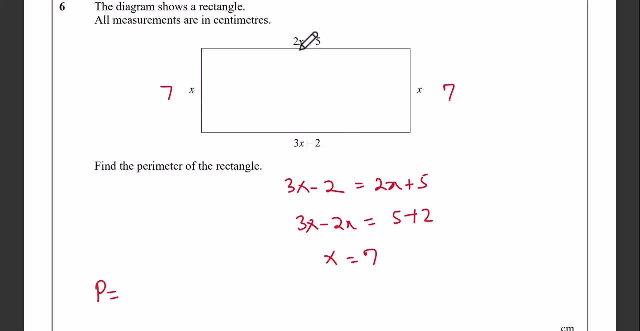 And here also is x, here is 7.. And the top has to be 2 times 7.. That's going to be like 14.. All right, And add 5.. That's going to be like 19.. And the down also was going to be 19 centimeters. 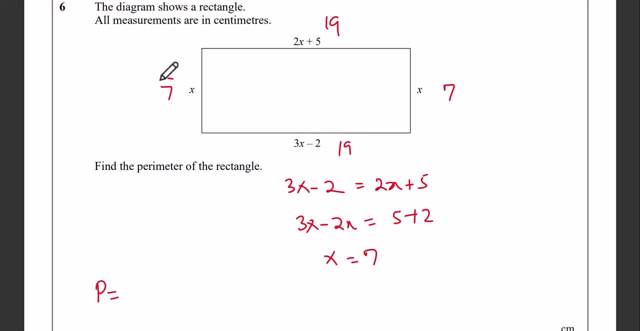 So to get the parameter, I have to multiply or add 7 plus 7 and add 19 plus 19.. So I add 19 plus 19 plus 7 plus 7.. Okay, Okay, Of course we add 19.. 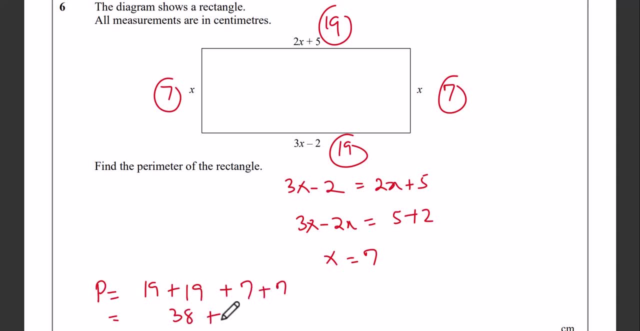 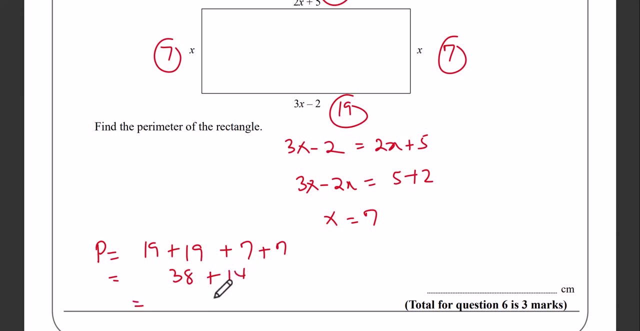 I think that's going to be. That's the 8. And that's 7.. So that's 14.. And, of course, if you add this, All right, I think this is going to give you like 180 is 12.. 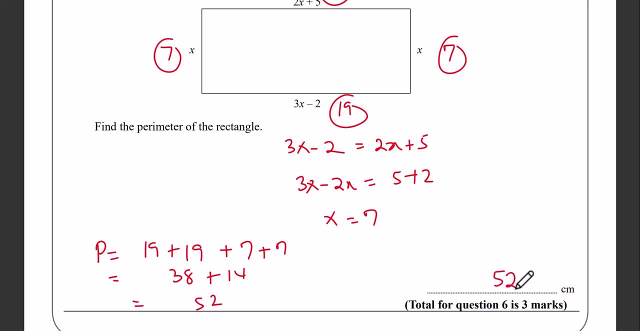 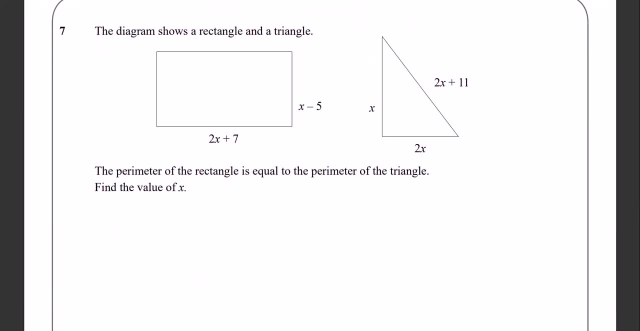 Carry 1 for 52.. So the parameter has to be 52 centimeters squared. And the next question: we have a triangle and a rectangle And we know that the parameter of the rectangle is equal to the triangle. They have the same parameter. 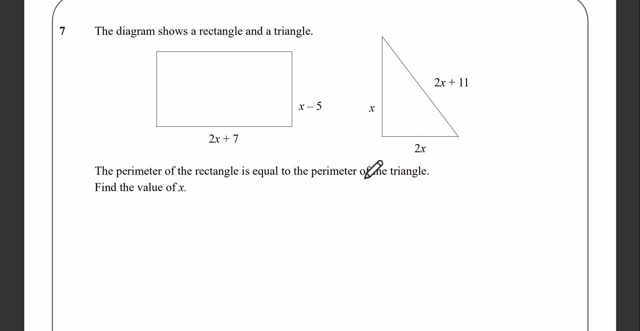 So we want to work out the value of x. All right, Now, one thing you can do, you can work out the parameter of the triangle. Yeah, quite easily. The parameter of the triangle is quite easy to get first. So if I add the parameter of this, it's going to be x plus 2x plus. 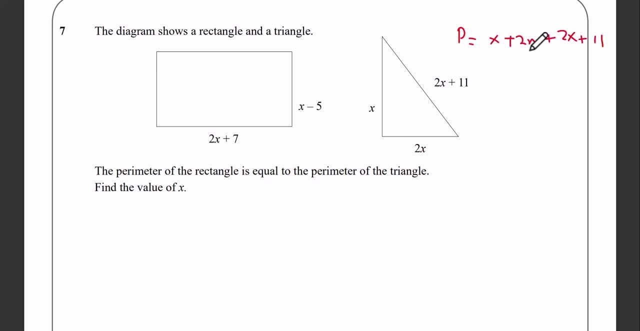 2x plus 11, right? So 2x plus x is 3x And of course here it's plus 2x plus 11.. And if you work it out, that's going to give you like. 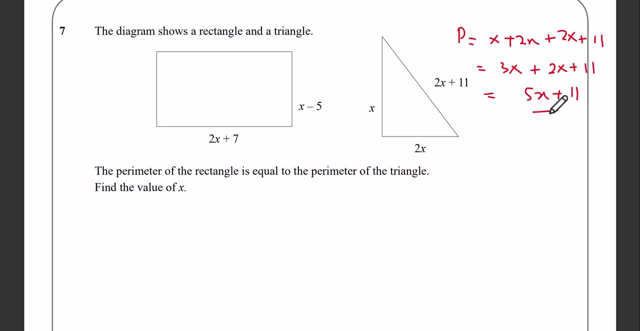 5x plus 11.. Now this here represents the parameter. All right, So we know that the parameter for the rectangle is the same thing as 5x plus 11.. And the parameter of the triangle is the same here. 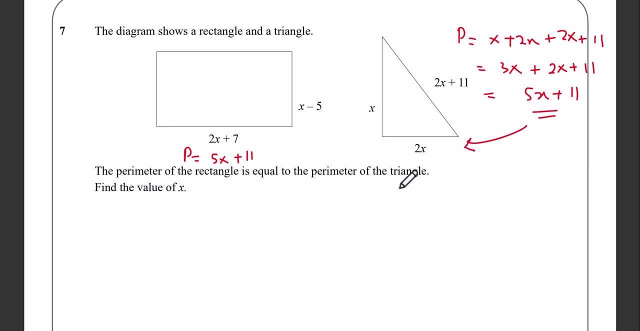 Okay, Good Now. so we want to work out the x Now. one of the way to work out the x is this: Because the parameter of the rectangle is equal to the parameter of the triangle. So you want to work out x. 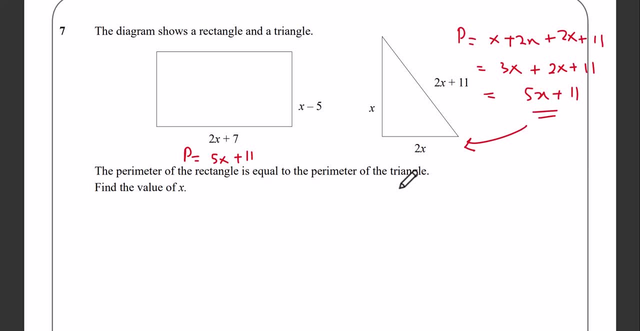 So I think what you needed to do is you may want to work out the, the parameter of this one here, Which, again, here's going to be: here's x plus 5.. x minus 5.. So here's x minus 5.. 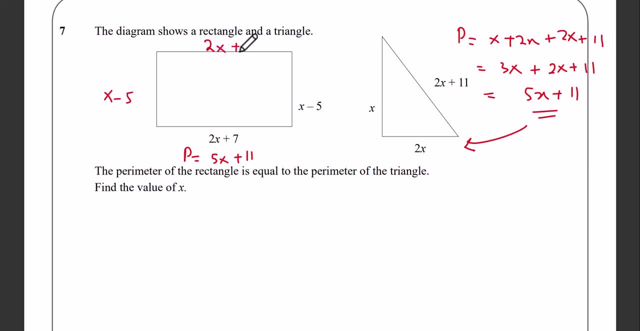 And here's 2x plus 7.. So the top has to be 2x plus 7.. And then, of course, if you add up the parameter, write it. write it like this: 2x minus 5.. 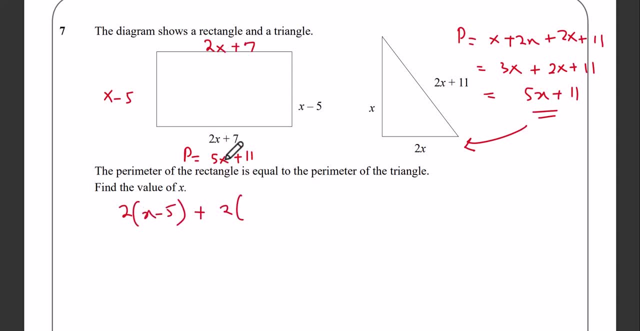 plus 2 bracket 2x. Oh, not 2x. Yeah, 2x plus 7.. Okay, For the parameter of this, And equate this to the original parameter Here, Which is actually 5x plus 11.. 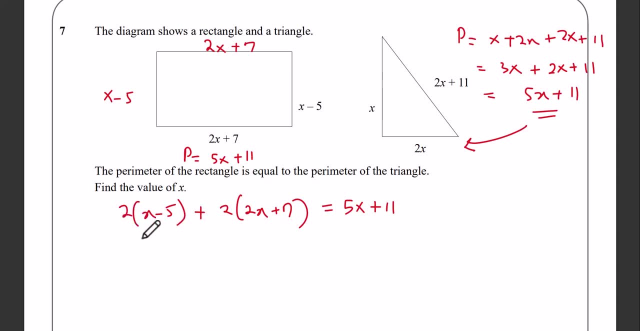 Alright, So let's work this: There's 2x minus 10. And that's 4x plus 14. And that's going to be 5x plus 11.. So 2x plus 4x is 6x. 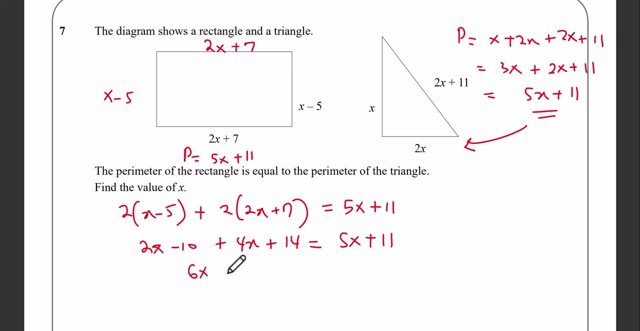 And minus 10 plus 14 is just going to be plus 4. And that's equal to 5x, And that's equal to 5x plus 11.. Of course, take away 5x on both sides, So that's going to be x. 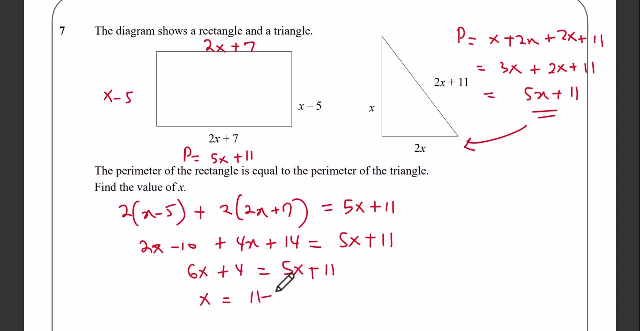 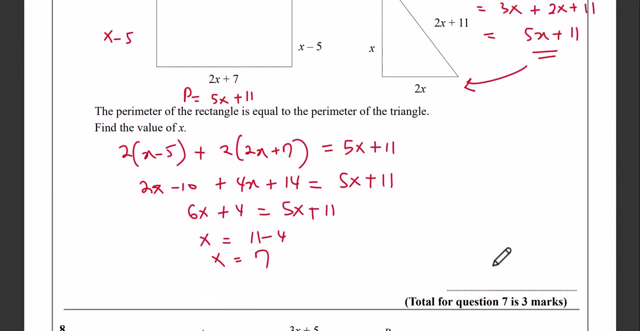 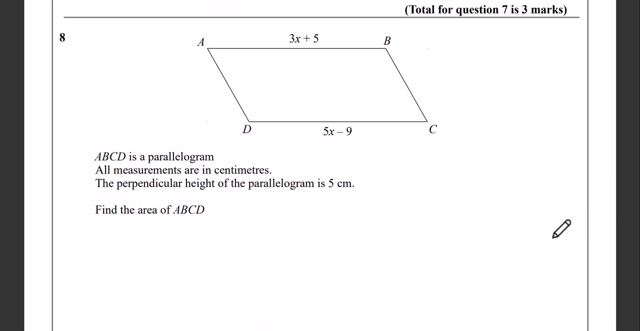 And subtract 5 on both sides, 11.. Take away 4.. So x is going to be like 7.. So we have looked at the value of x. It's definitely going to be 7.. And we come to the next one number, 8.. 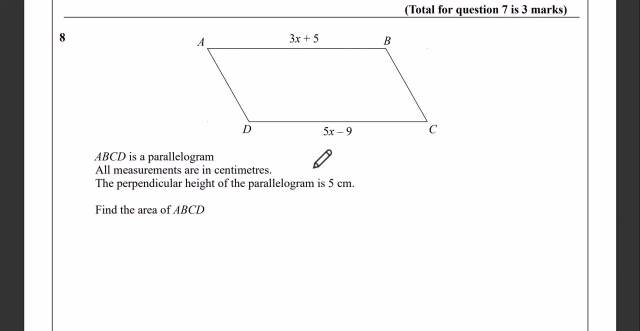 We have a parallelogram ABCD, And all measurements are in centimeters And the perpendicular height between the two parallel lines- Yeah, the height here, The vertical height, is 5cm, So we need to work out the area. 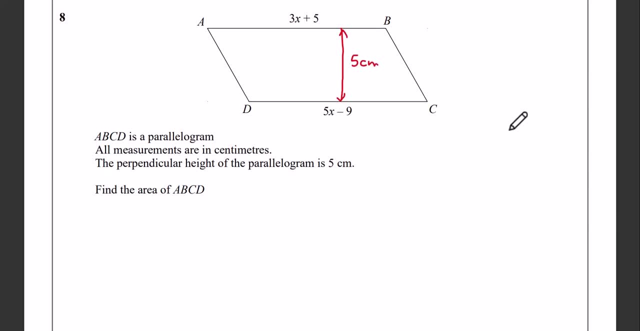 Now, of course, you know, the area of a parallelogram is the base times the perpendicular height. Okay, Good, So we know the height, which is 5.. But we don't know the numerical value of the base. But we can work that out by doing the same thing here. 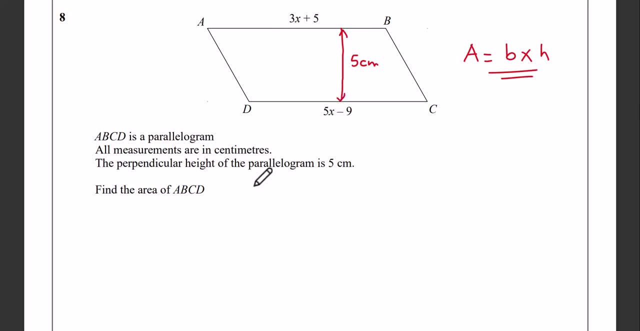 This is equal to this side? I think so. Yeah, So 5x minus 9 is the same as 3x plus 5. And of course, subtract 3x on both sides, That's 5x minus 3x. 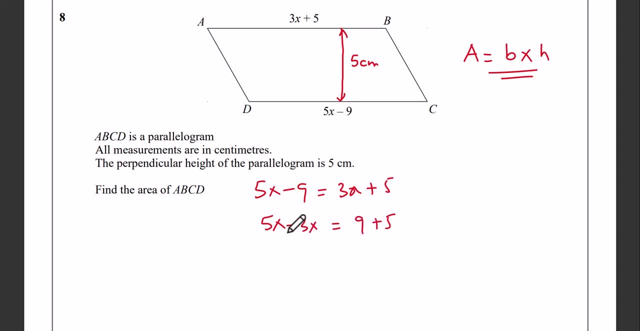 And add 9 on both sides, That's 9 plus 5. And if you simplify further, you get 2x And you get 14.. So x is definitely going to be 7.. Okay, So by 2.. 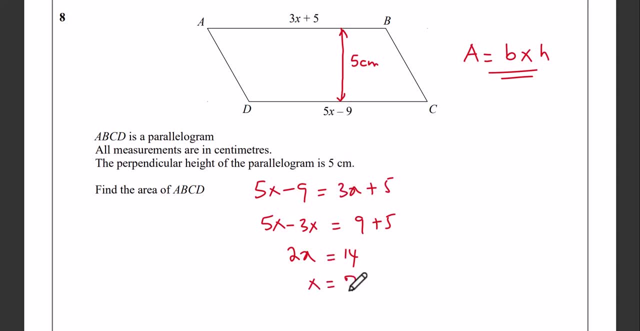 So that means if x is 2,- I mean x is 7, then of course you can work out the value for either the bottom or the top. So that means if I substitute x here with 7,, 5 times 7 is 35.. 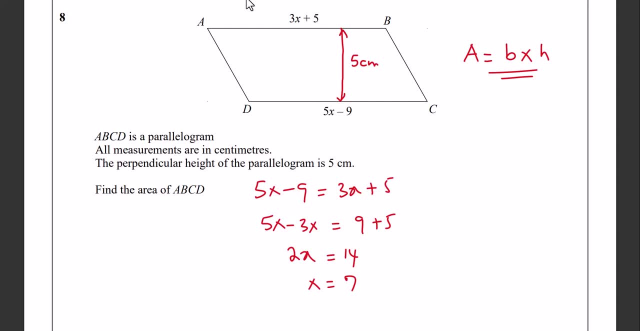 Yeah, So if it's 35 minus 9,, what do you get? You get 26.. Yeah, So this is 26 for the base. So the area is definitely going to be the base, which is 26,, and times it by 5, the 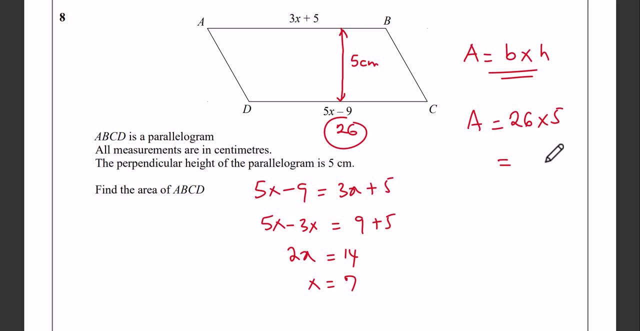 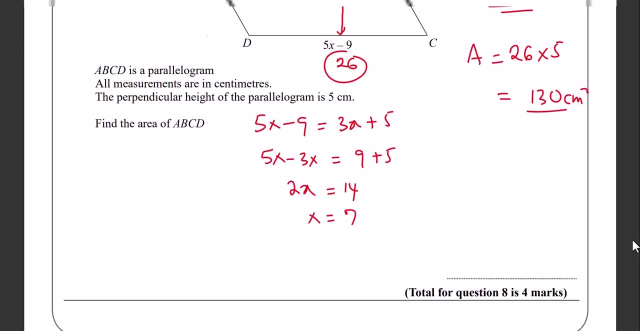 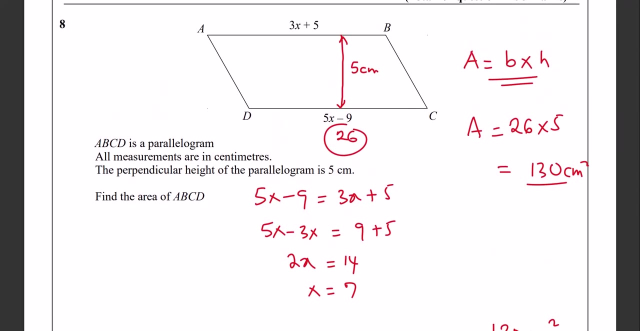 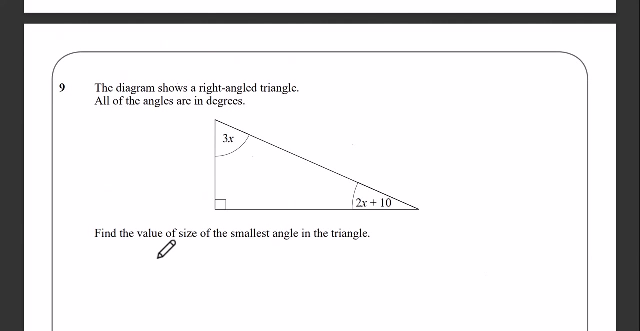 height And that's going to give you like 130 centimeters squared. So the area is 130 cm squared. We have one here, We have another triangle And you don't want to work at the smallest angle possible. 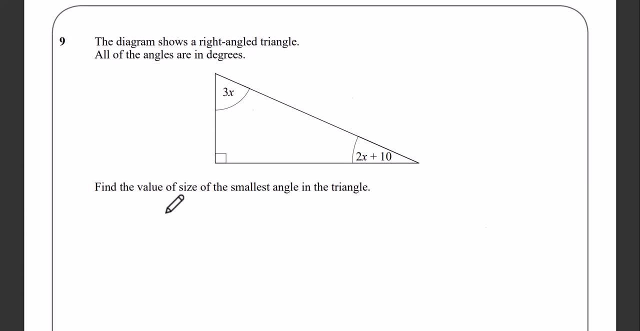 I think what you can do is add up all the angles in the triangle And 2x plus 10 and angle 3x And then 90, because this is 90. Of course, if you add up all the angles in the triangle, they give you 180. 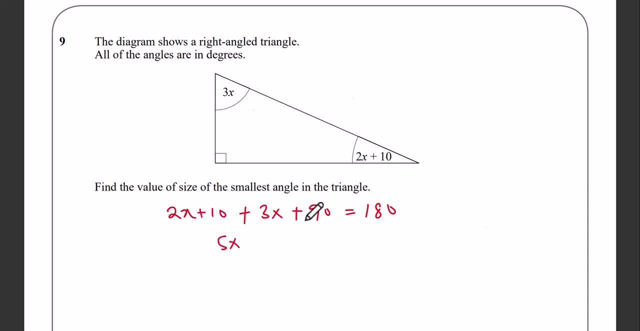 So 2x and 3x is 5x, And 10 plus 90 is 100.. 100 equals 180.. And subtract 100 from 180.. So 5x is going to be like 80.. 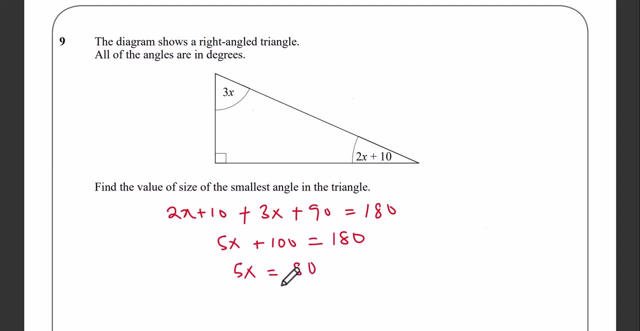 Yeah, Good, And now you have: 5x equals 80. So x is definitely going to be like 16.. Divide 80 by 5, you get 16.. Okay, So that means this 3 times 16 is going to give you like 3x. 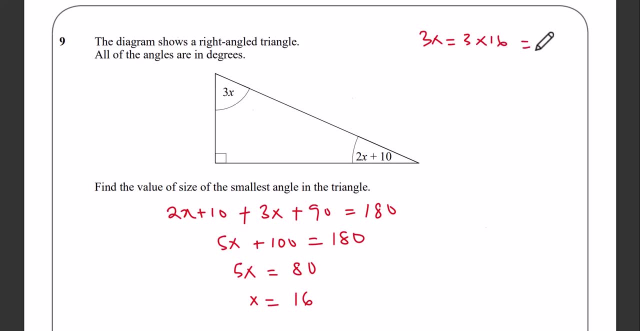 Which is 3 times 16.. That's 48.. So this whole angle here is 48 degrees And this other one, which is 2x plus 10.. 2x plus 10 is going to be 2 times 16.. 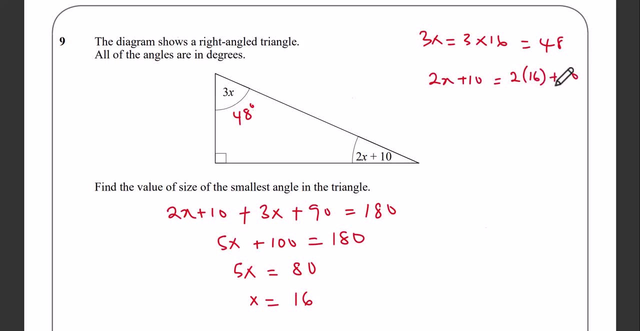 And add 10 to it, That's 32 plus 10.. 32 plus 10 is 42.. So this angle is 42.. I think that here is 90 degrees, So obviously the smallest angle has to be this one here. 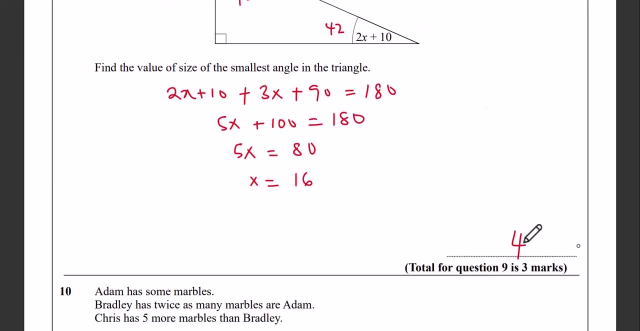 Which is 42 degrees. Yeah, So I think this is how far we can go on this And thank you so much.